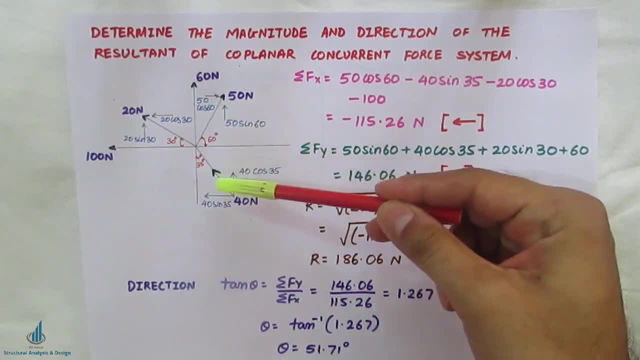 So what you have to do is, wherever this inclined force is there, we have to split this forces into horizontal component and vertical component. So this 50 Newton I have resolved into horizontal and vertical component. But the main important aspect is where to write sine and cos, The 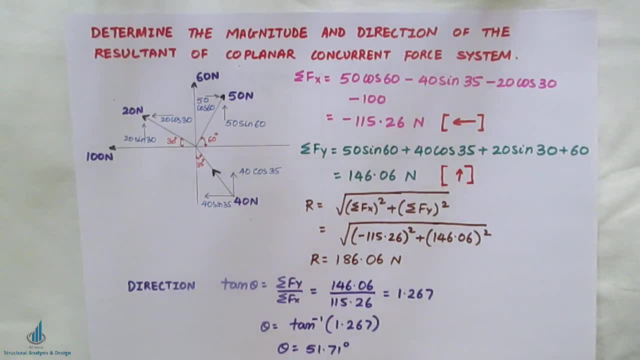 students usually gets confused to write sine and cos. So the important instruction I will be giving is: whatever the component is sorry, wherever this degree is means theta, opposite to theta. whatever the force may be that you have to write as sine Understood. Whatever the component is there, opposite to that particular. 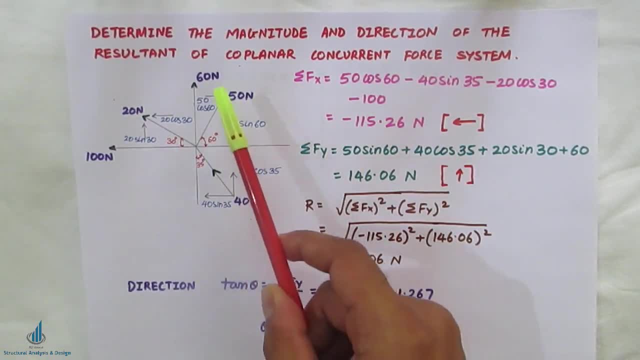 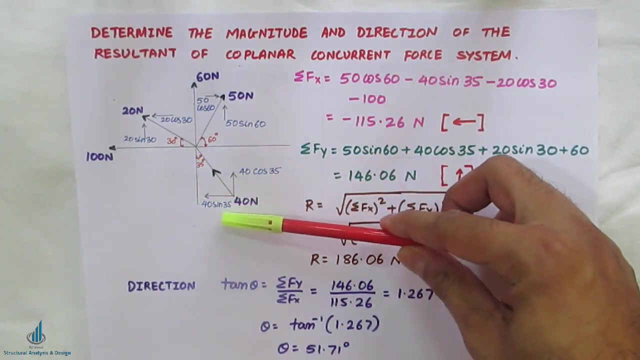 theta, you have to write it as sine component and the remaining will be the cos component. Similarly, see here the 40 Newton is acting at an angle 35 degrees. So this theta, opposite to this theta, is horizontal component And the opposite will be the sine component. Don't remember that opposite to theta will be always. 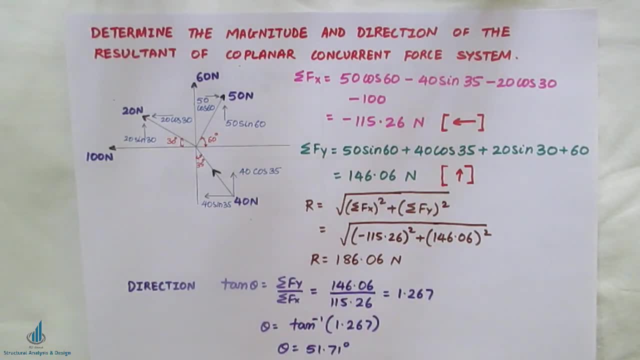 vertical or it will be always horizontal. No, Okay, So be specific, that opposite to theta will be your sine opposite and the other remaining will be the cos. Similarly, for this 20 Newton force, opposite to this, 30 degrees, is horizontal- sorry, vertical- component, and I have written it as sine component. 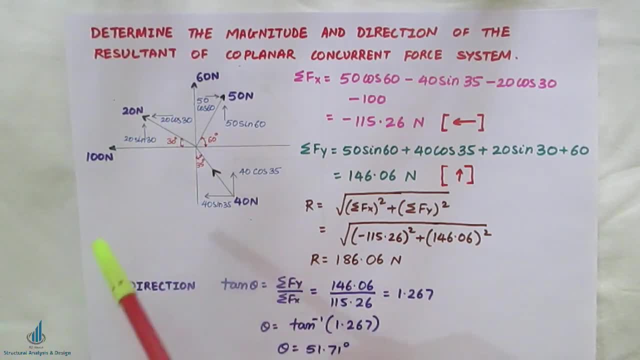 and the remaining will be the cos cos. and don't remember that always it will be horizontal or always it will be vertical. it depends upon the component of that particular with respect to that opposite theta. okay, so sigma fx. sigma fx is nothing. but whatever the force is acting in the x direction, whether it may be, 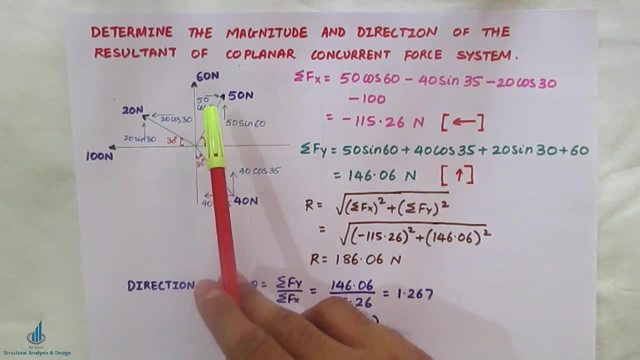 positive or it may be negative. so the first component will be 50 cos 60. okay, this horizontal component, which is x, 50 cos 60, it is moving in the right hand side direction, so it is positive. next will be 40 sine 35. okay, so it is moving in left hand side. so that's why i've 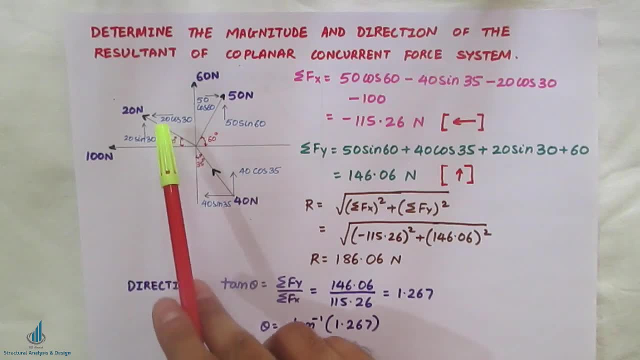 written here: minus 40 sine 35. next will be 20 cos 30. again, it is moving in the left hand side direction. so minus 20 cos 30 and the remaining, okay, which is the straight component which is not in inclined. you need not have to split this component. okay, so directly: minus 100 because it is moving. 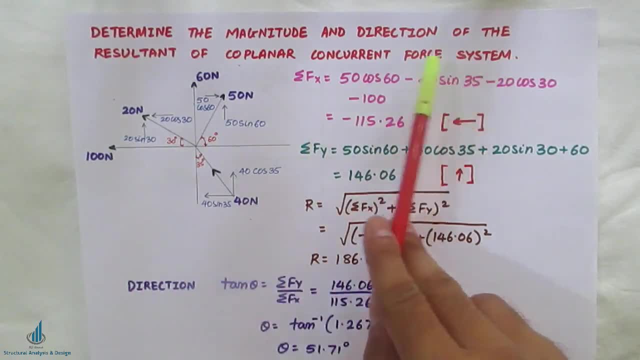 in left hand side direction. so whenever you do this particular calculation- okay, based on the direction of x direction, so you'll be getting this- sigma fx is equals to minus 115.26 newton for this particular force system. once again, i will repeat: plus 50, cos 60, minus 40 sine. 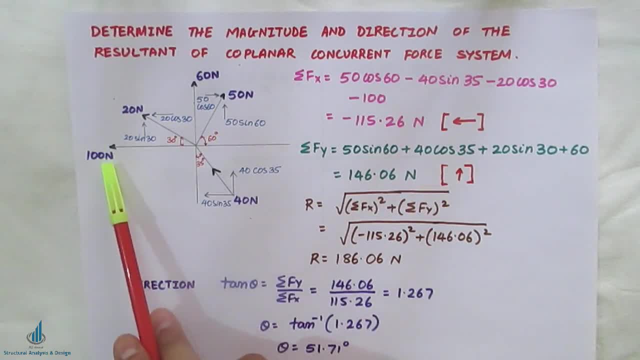 30, 35 minus 20, cos 30 and minus 100, based upon the direction of x. okay, similarly, you have to find out sigma y, the summation of y components or vertical components. so this one will be 50 sine 60, because it is moving in positive direction or upward direction. okay, upward direction will be. 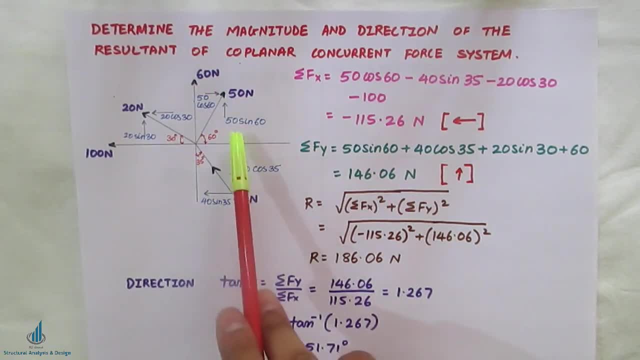 positive downward direction will be negative. so it is moving in upward direction. so 50 sine 60, next again it is moving upward, 40 cos 35, again it is moving uh upwards, for 20 sine 30 and the last one which is not inclined here, only 60, no horizontal or no vertical again. you have to split up, okay. 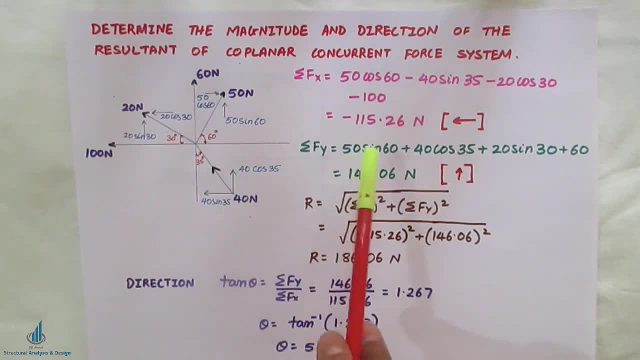 directly, you have to take 60, because it is moving in positive direction. all components are positive, so the calculation will be 146.06 newton in positive direction. i have mentioned here minus means it is moving left hand side direction and the vertical is uh 146.06 positive, so upward direction. so the resultant is given by the formula square root of: 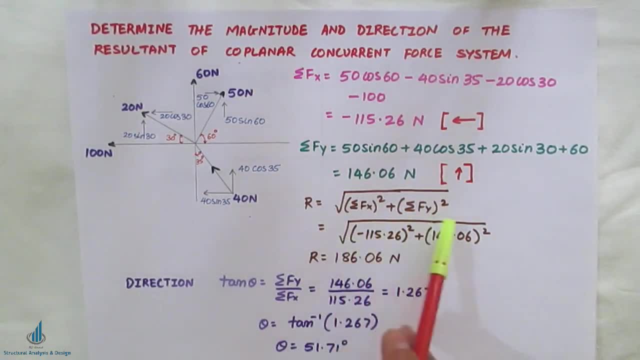 sigma fx, the whole square plus sigma f by the whole square. after substituting the sigma fx and sigma f, i will be getting the resultant 186.06 newton. so the resultant of this particular force system is 186.06 newton, and direction is nothing but theta. okay, at what angle this resultant will?